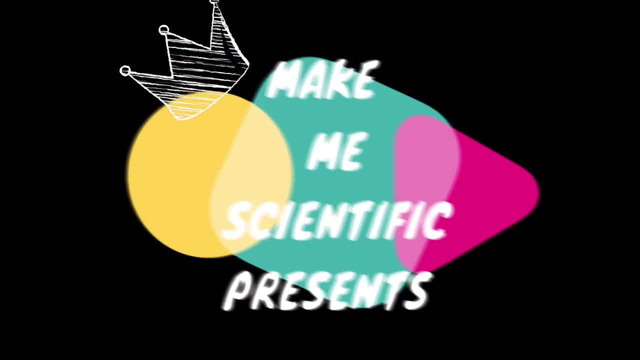 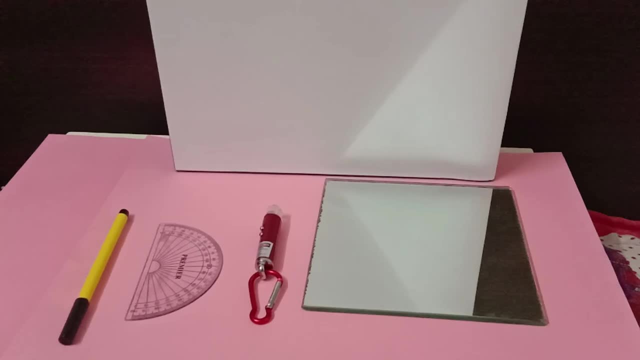 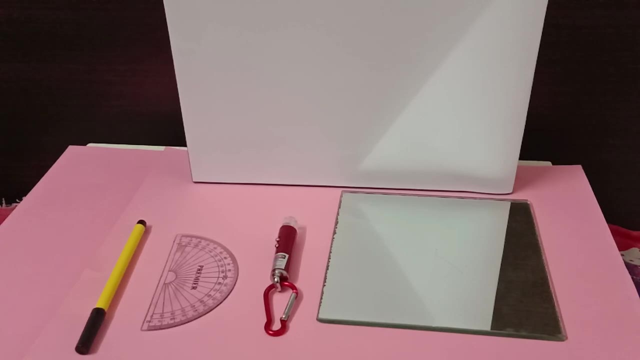 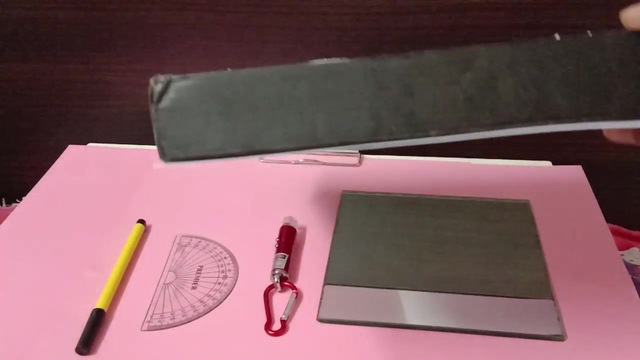 Hello scientific audience, How are you all? So today I am going to demonstrate the laws of reflection of light by using a laser protractor, some basic stationary plane mirror and the screen. So screen is nothing but a white background. So I had a small piece of cardboard. 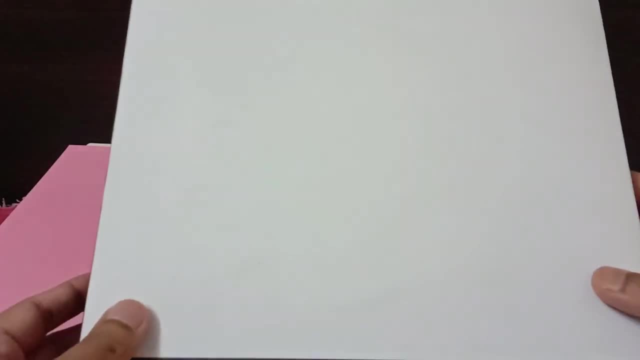 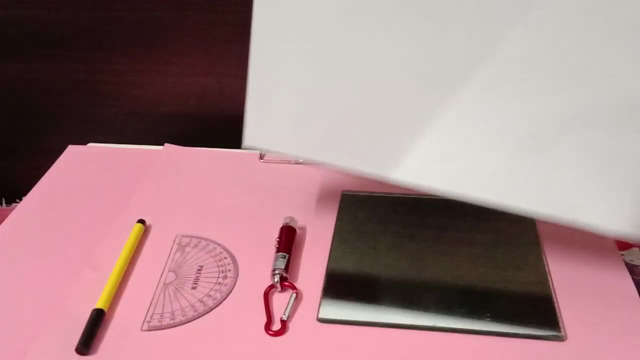 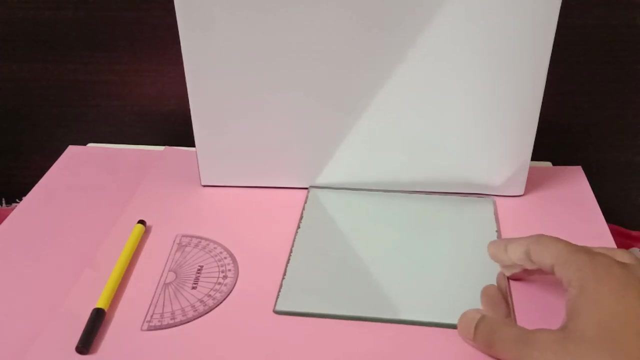 on which a small box on which I have attached a white A4 size paper. So this is going to act as our screen. Now what happens is: this is the mirror, and the first law states that incident ray, reflected ray and normal they all lie on the same plane. So that can be. 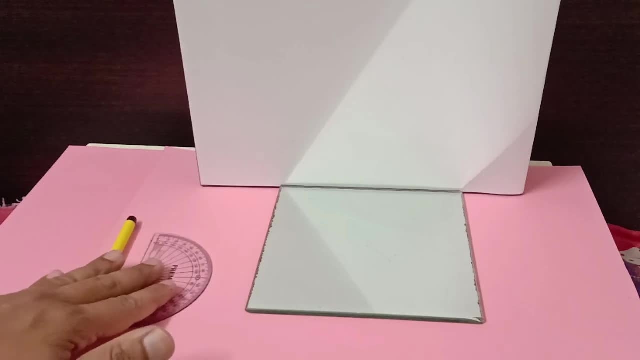 easily demonstrated even without the use of the protractor. and you will understand why we are using protractor, because the second law states that the angle of incidence and the angle of reflection are same. So we need to prove that. So here I am going to use 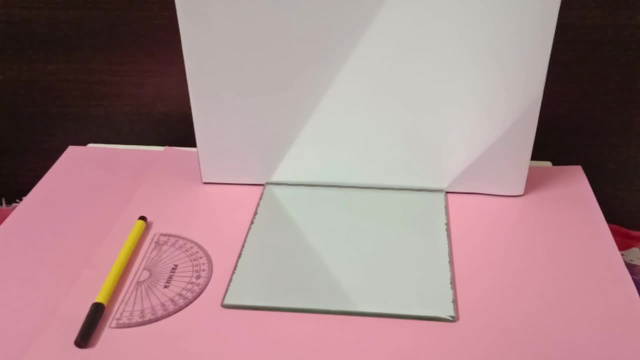 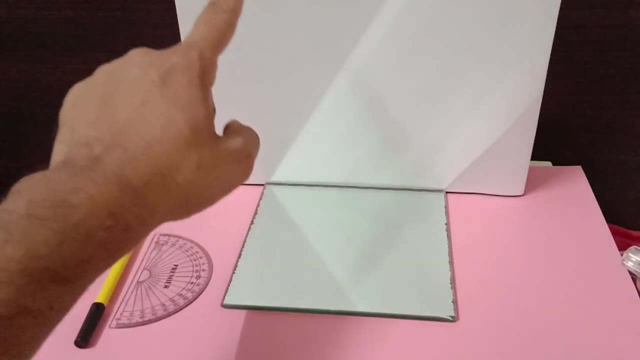 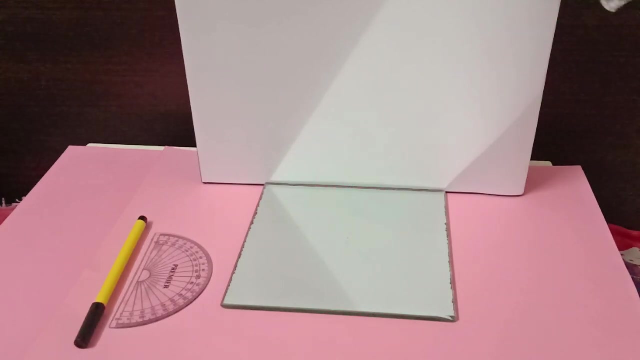 a red laser right in order to support my demonstration and anything. So what you see in the mirror will be the reflection We are supposed to concentrate on this white screen. Okay, So this is our incident ray. The incident ray is this one. 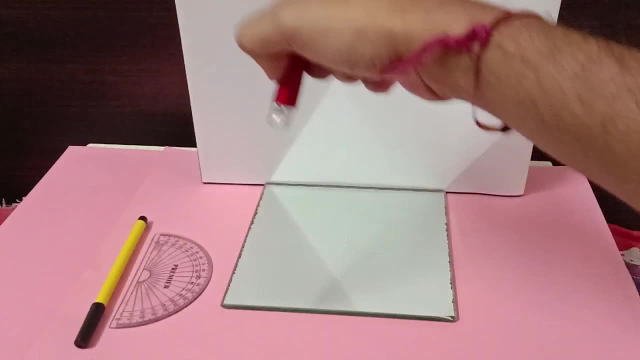 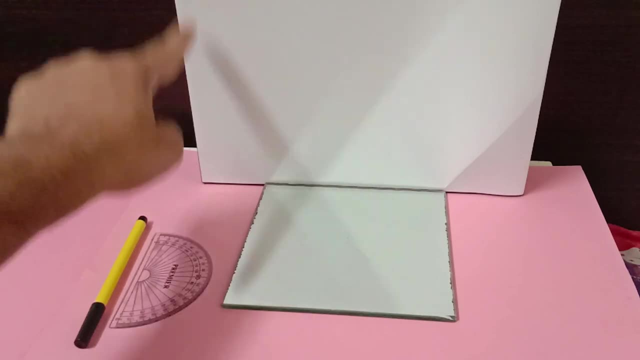 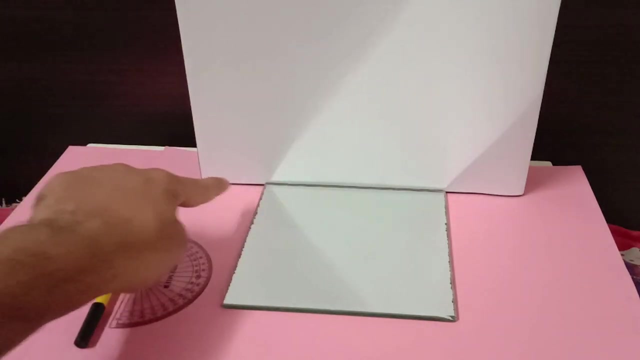 which is seen over here, and you will see that the reflected ray will also be on the, on this particular white screen. So this white screen is nothing, but you can consider this as y-axis, this as x-axis and this will be z-axis towards us. So this white screen is nothing but xy. 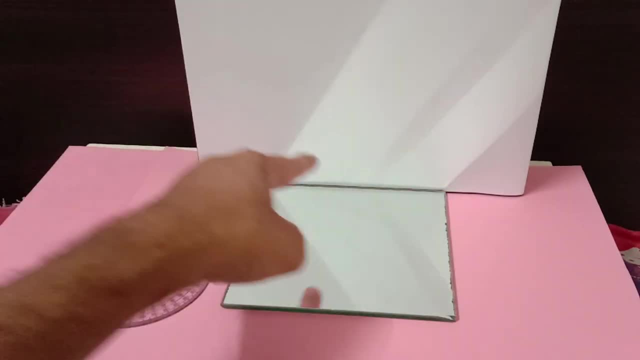 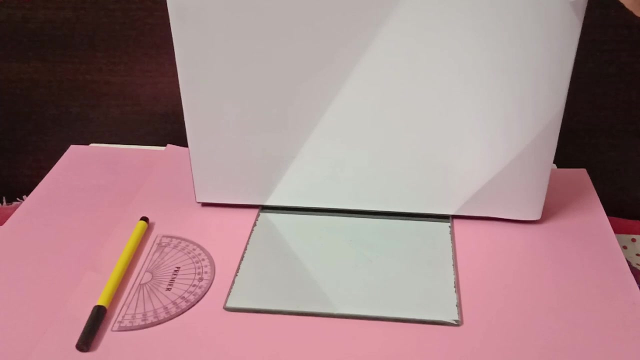 plane and the incident ray and the reflected ray would definitely be on the xy plane and from here, if you draw the normal that separates both incident and reflected ray, you will see that all three will on the same plane here. So I am shining the red laser from. 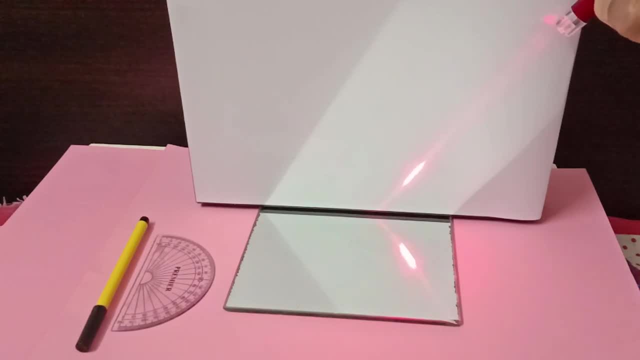 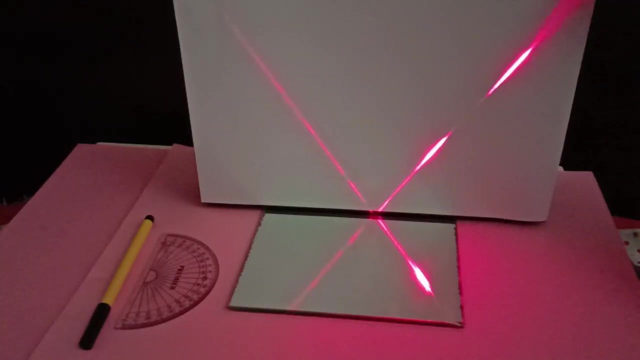 this side and you can clearly see the incident ray and the reflected ray as well. So incident ray, That is the reflected ray, and the normal is here and you can see that all three lie on the same plane. To have a better view, I have switched off the light in the room and now 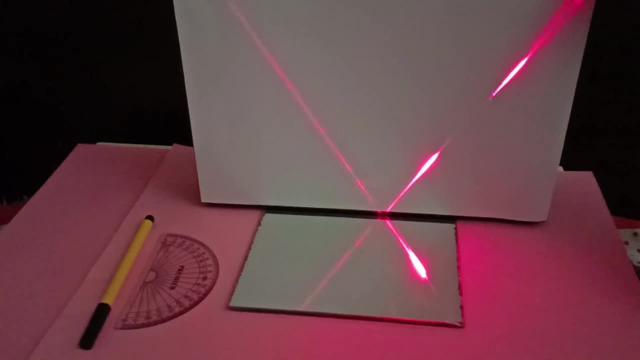 this is very well visible, that this is our incident ray, that is our reflected ray, and here is our normal and this point where the laser light would strike on the mirror, that would be the point off. So this is the angle of incidence right Now. unfortunately, I do not have another. 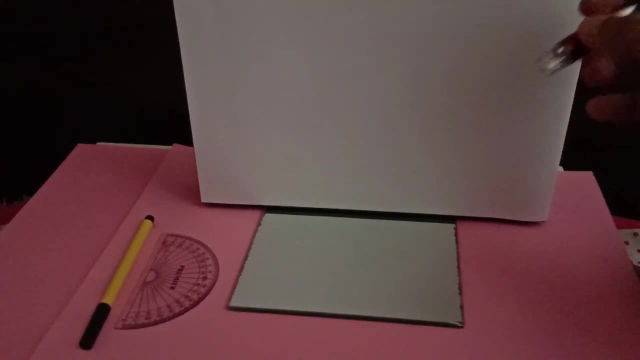 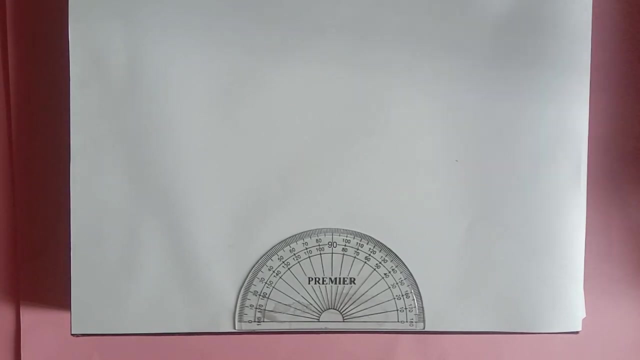 stand so that I can hold this laser. So I am doing it by my hand, So the point of incidence may keep on changing, but hopefully the idea is you have understood. Okay, so we are good to go for the second law of reflection, that is, angle of incidence. 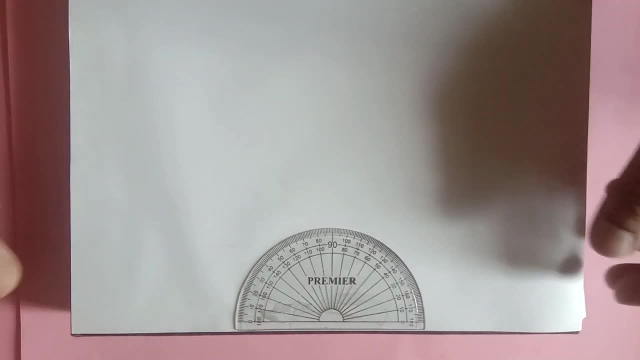 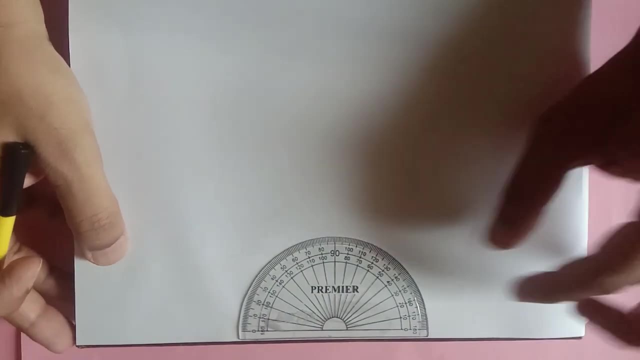 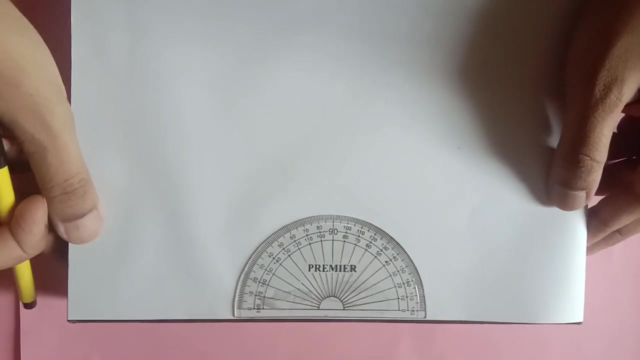 is equal to the angle of reflection. and what I have done is the same cardboard box on which I had fixed This A4 size paper, and now I have also fixed the protractor on this white A4 size paper, so it does not move with the help of a glue, right? Okay, now what my plan is that this: 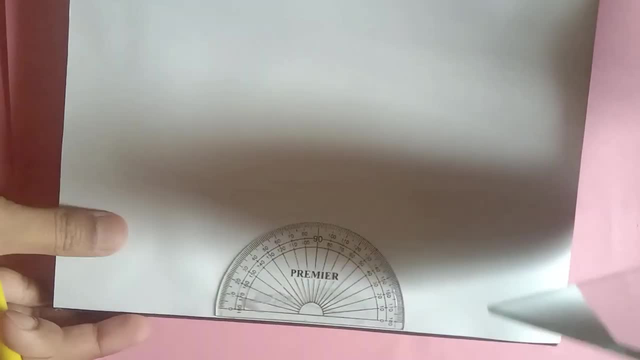 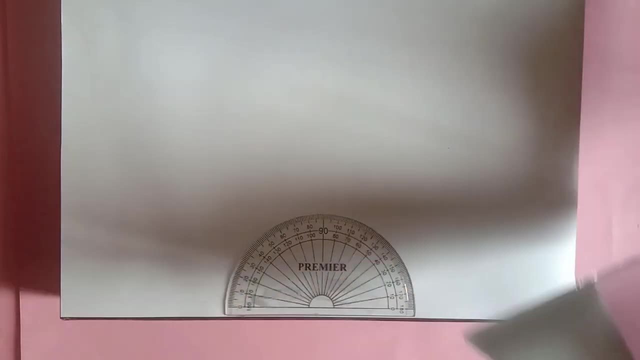 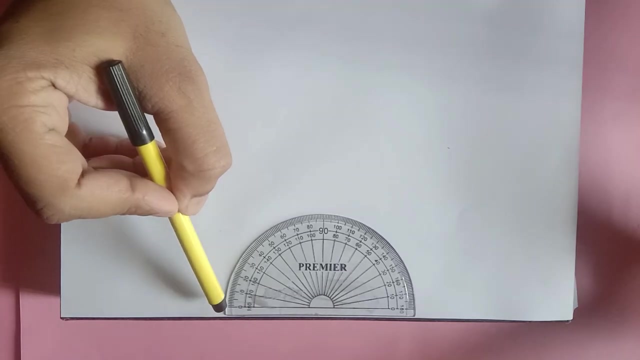 is my plane mirror, and this plane mirror I am going to arrange perpendicular to this plane of paper, correct? So I am going to put it somewhere here on the protractor and I would make sure that this, This plane mirror, is perpendicular to the plane of paper and along this line, right? 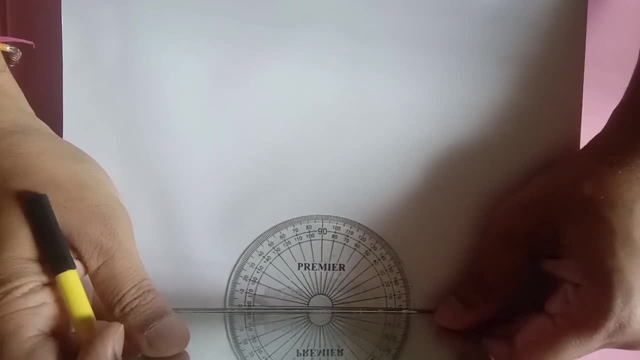 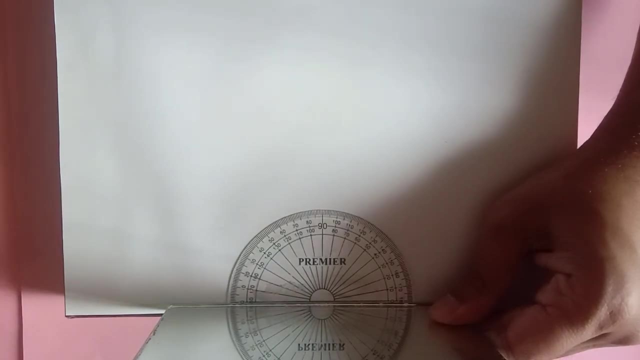 Like this, and now I would make sure that this mirror does not move. So I will, I will hold this mirror rigidly Now I will pass the incident ray through here, So it would strike the mirror and it will go somewhere like this. So this would be my target point. Okay, so, 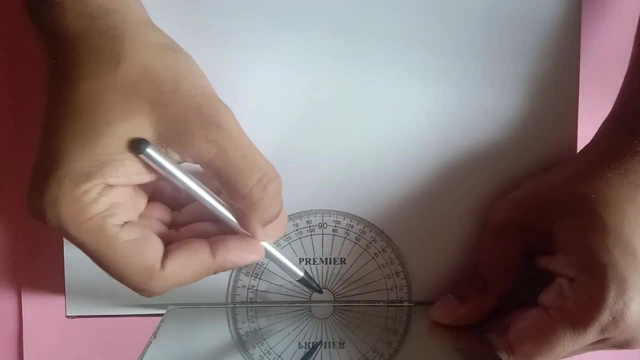 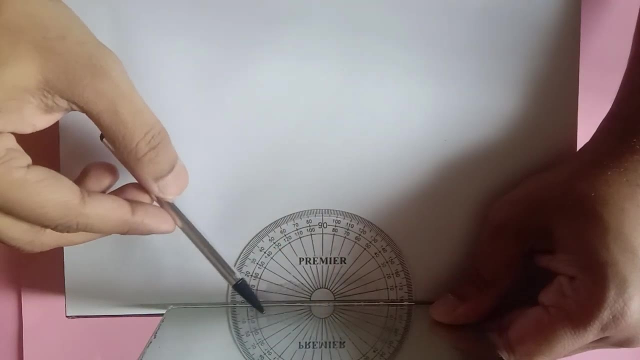 this is my target point. I am planning to incident the light at this point, exactly at the middle point over here. So that would become the point of incidence and this would be the direction of my incident ray. So incident ray would pass from here, It would strike.